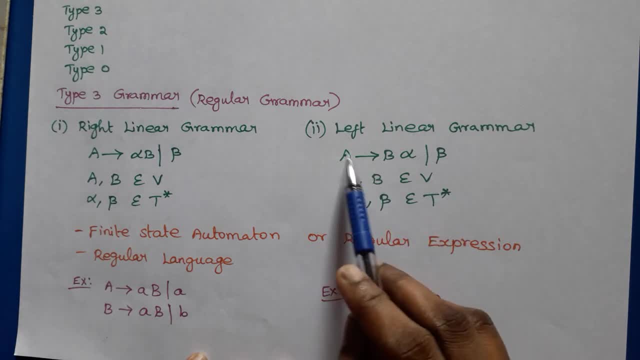 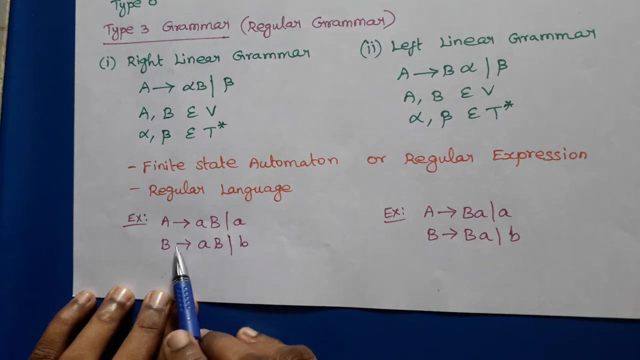 that is, any number of. So a variable tends to string of terminals, or a variable tends to variable followed by string of terminals. For example, in this grammar a tends to a, b bar a and b can be expanded like this, So a can be replaced by a, b or simply a. Suppose if we have to consider this. 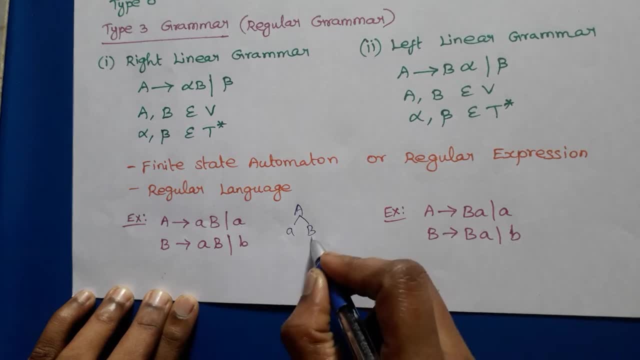 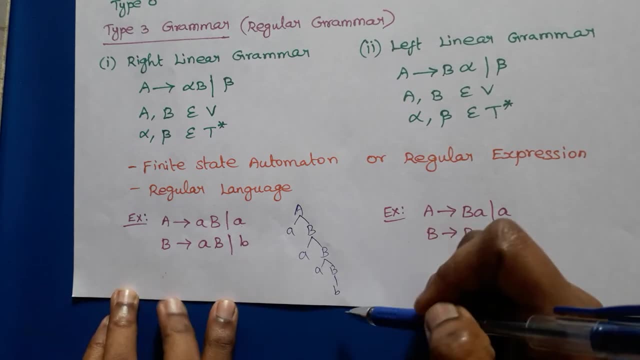 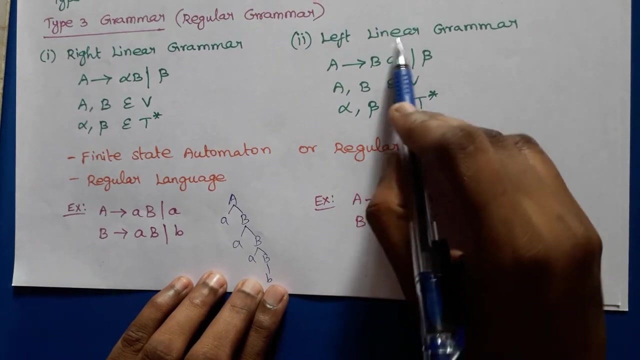 production. a can be replaced by a- b. So a can be replaced by a, b any number of times. Finally, it should be replaced by b. Okay, so we will get. it is expanded like this. Therefore, it is called as right linear grammar, If we. this is the example for left linear grammar. So here a variable followed by a. 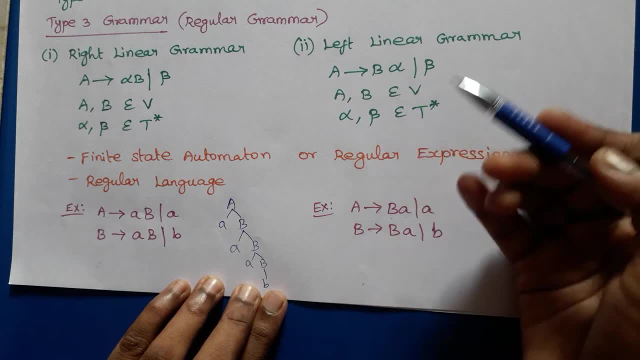 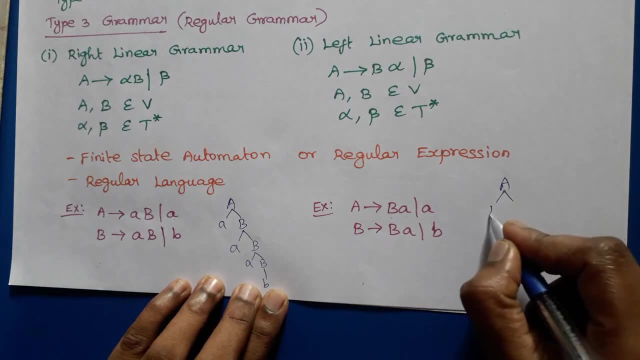 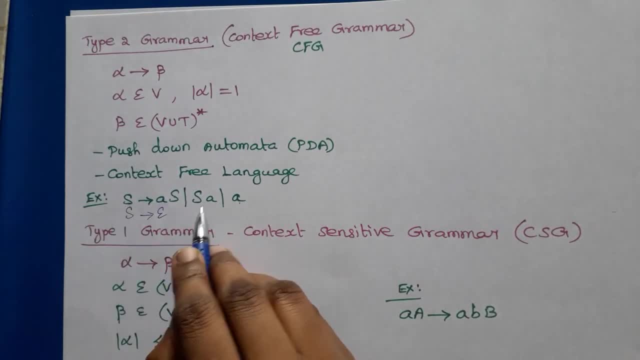 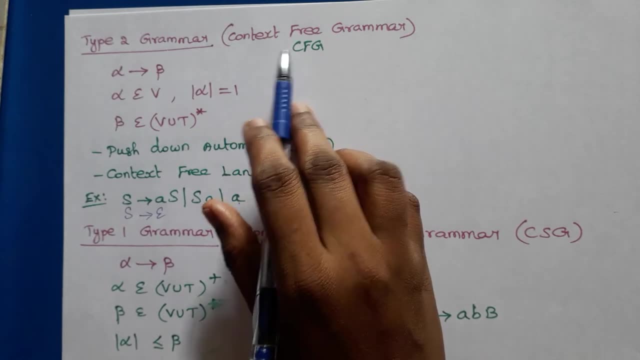 write a parse tree for this. So we can write a parse tree for this. So we can write a parse. wherever s appeared in the string, it can be replaced by the body of the production. okay, that it won't depend upon the context. therefore, it is called as context free grammar, for example: 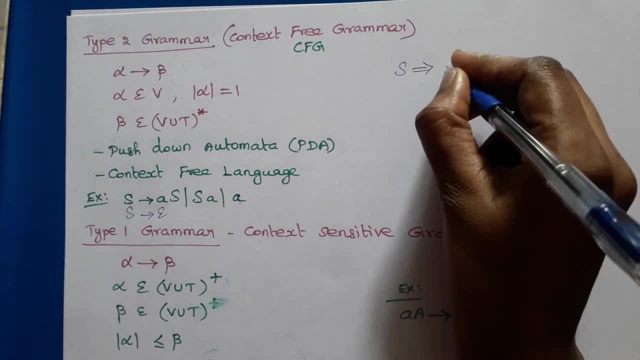 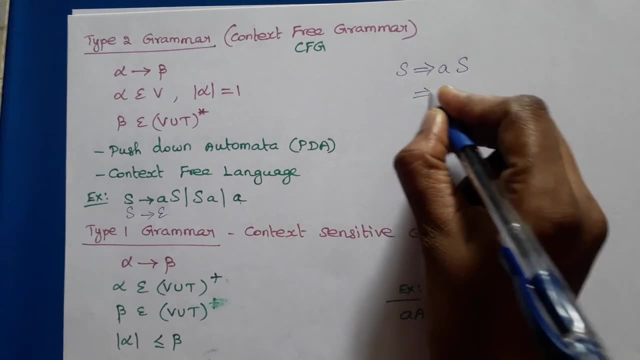 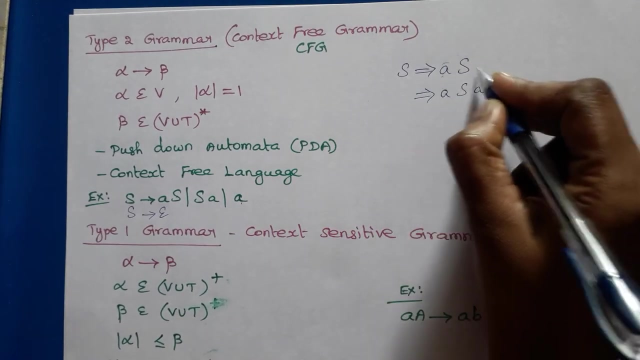 we can derive this like this s can be. s appears here, so it can be replaced by any one of the production. and in the next step, also, s can be replaced by any one of the production. okay, here, this is the context- means the nearby symbols. we don't worry about the context, the previous or 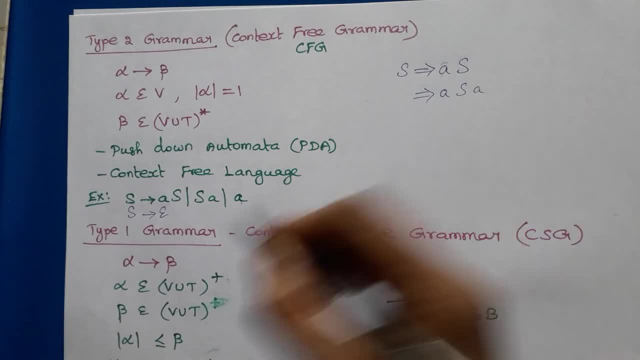 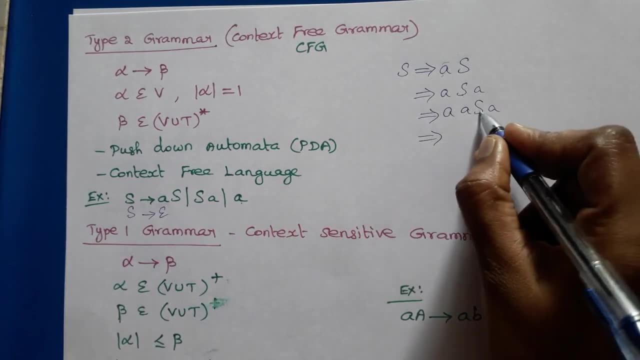 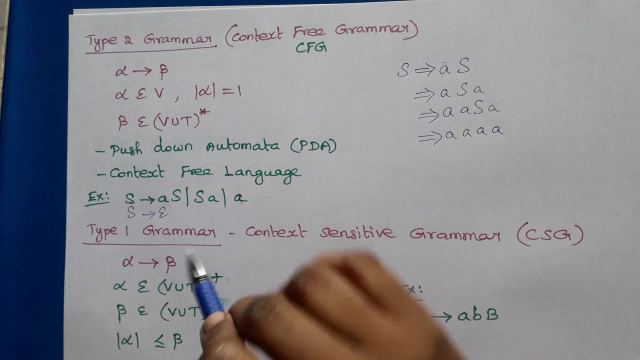 following symbols: wherever s appears, it can be replaced by any one of the production and in the step, it can be replaced by a s, and this s can be can be replaced by a. okay, therefore, it is called as context free, but context sensitive grammar means we will consider the context also. 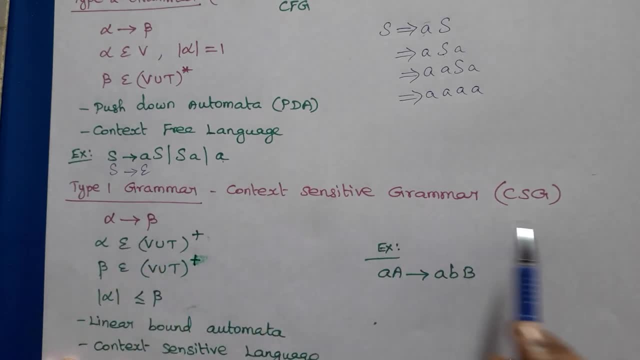 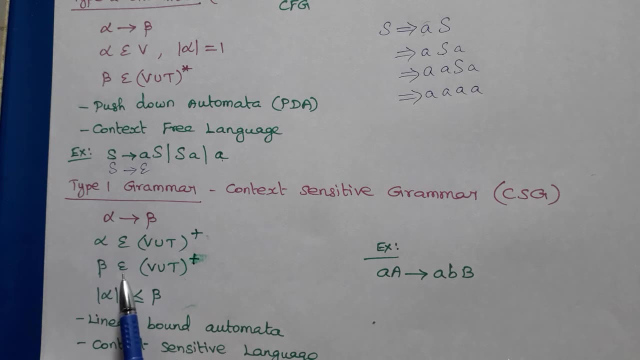 okay then. type 1 grammar is otherwise called as context sensitive grammar, CSG. here also all the productions are in this form: alpha tends to beta, where both alpha and beta are one or more variables and non-terminal variables or terminals. So epsilon production is not allowed here, okay. 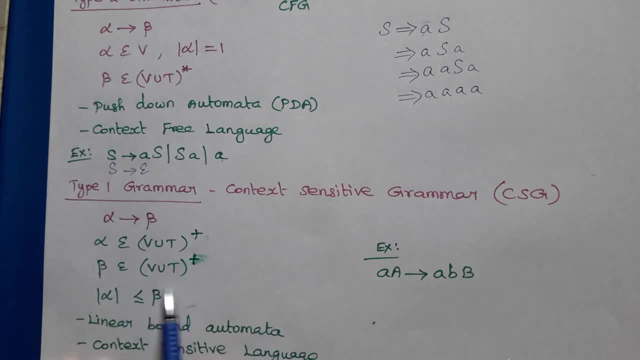 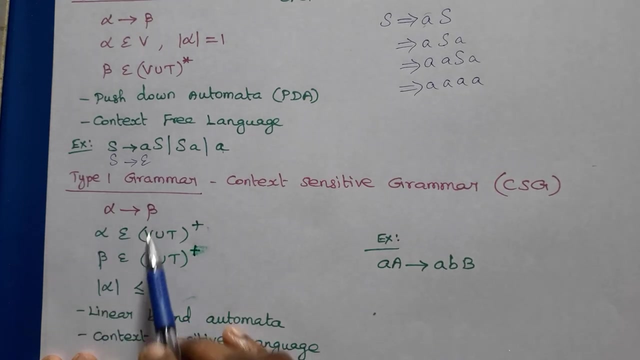 because beta should be at least one non-terminal one, at least one variable or terminal symbol. So epsilon is not allowed here. So, but here the restriction is alpha. length of alpha must be less than or equal to length of beta. For example, a, a tends to a, b, b, So here length of alpha is: 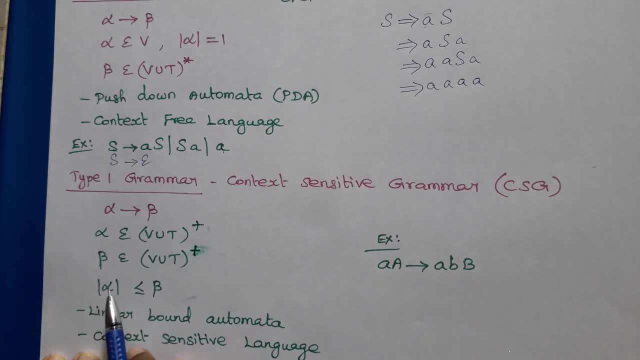 2. length of beta is 3. okay, always, length of alpha should be less than or equal to length of beta. So here a. a can be replaced by small terminal a and variable a can be replaced by this one. The meaning is a. if you want to replace, expand a. 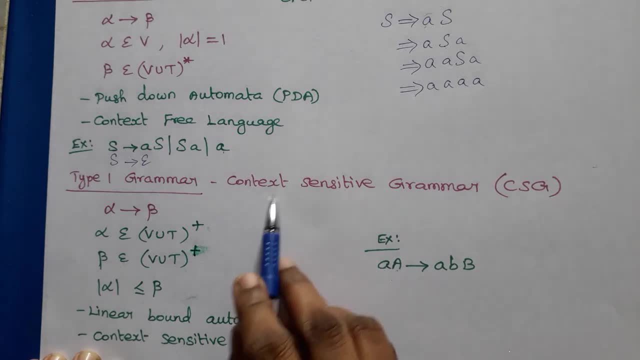 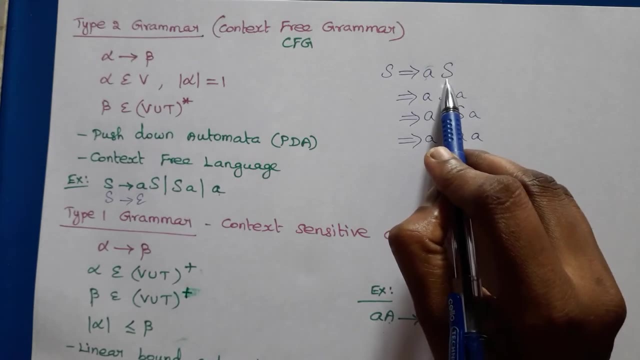 it should be preceded by the symbol a. So context. therefore it is called as context sensitive grammar. So if you want to replace here, if you want to replace s simply s can be replaced by any one of its productions. We won't worry about the preceding or following symbols. 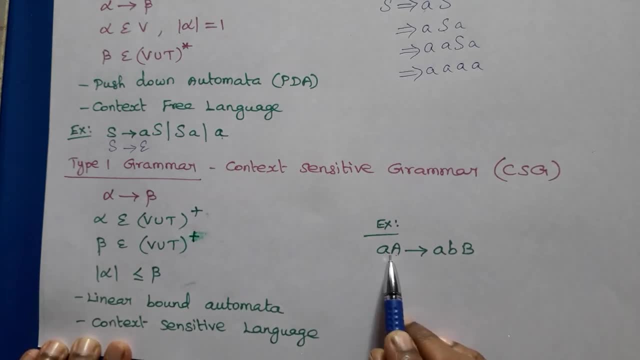 But here in this example a is preceded by small letter a, terminal a. So variable a is preceded by small letter a, So variable a is preceded by small letter a. So wherever a, a appears during the derivation, it can be replaced by a, b, b, For example suppose. 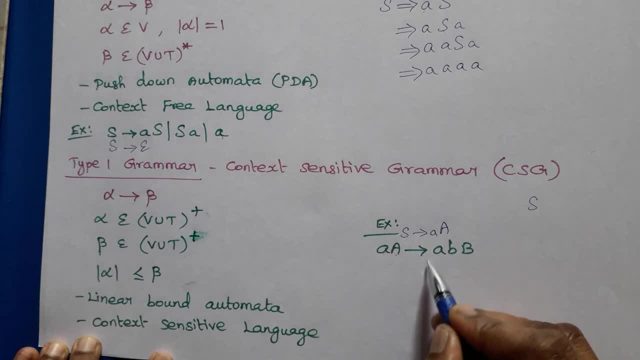 assume that this is considered as a grammar. So s can be replaced by a, a, and in this a is preceded by a, So the both symbol can be replaced by a, b, b in the next step. So a b, b like the. 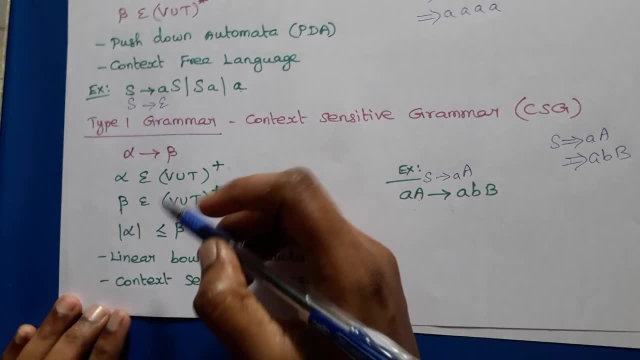 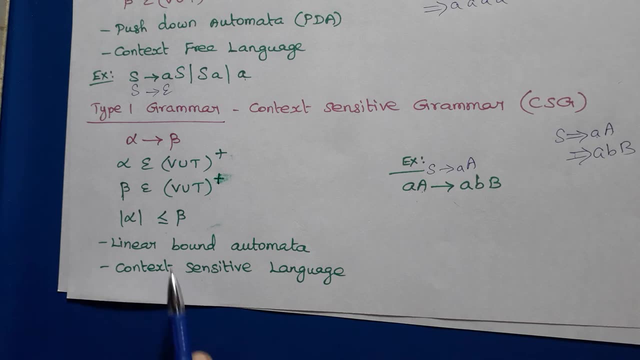 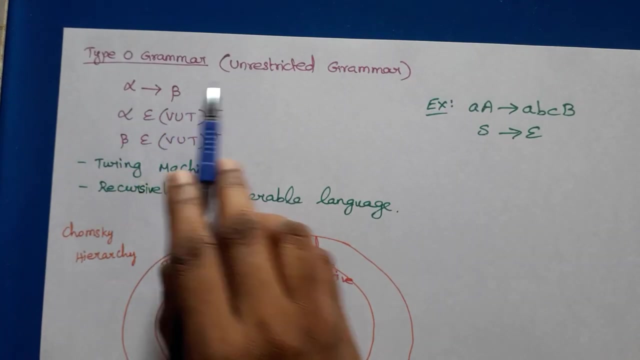 likewise. So this is called as context sensitive grammar, and the mathematical model that accepts this grammar is called as a linear bound automata, and language generated by this grammar is context sensitive language. Then the last one is the final one is type 0 grammar. This is unrestricted grammar. There is no restriction here. All the productions.